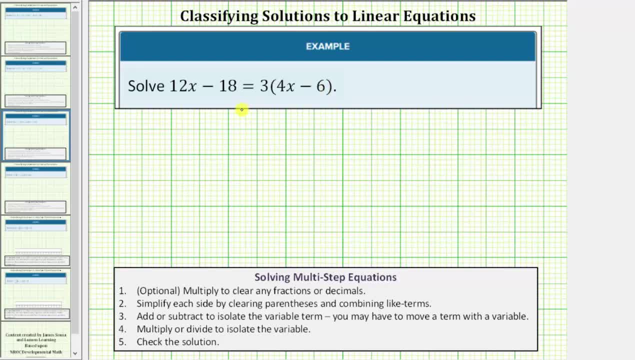 We want to solve the given linear equation in one variable. Normally, when solving an equation like this, we expect to have one solution, But that's not always the case. Let's try to solve this equation and see what happens. Following the guidelines to solve a multi-step equation, the first step would be to clear the parentheses on the right side of the equation by distributing three. 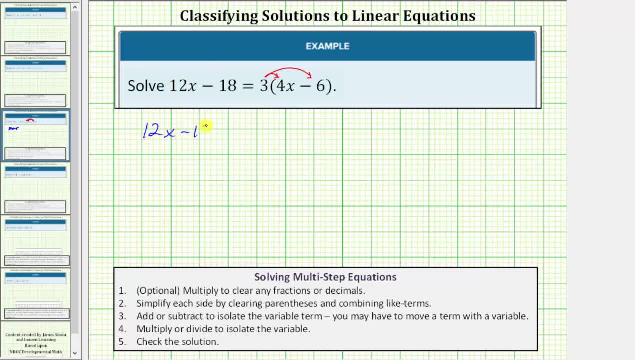 So the left side remains 12x minus 18.. Now on the right side, 3 times 4x is 12x. We have 12x minus 3 times 6 is equal to 18.. Now, looking at the equation closely, notice how the expression on the left is exactly the same as the expression on the right, which means any value of x is going to satisfy the equation or make the equation true. 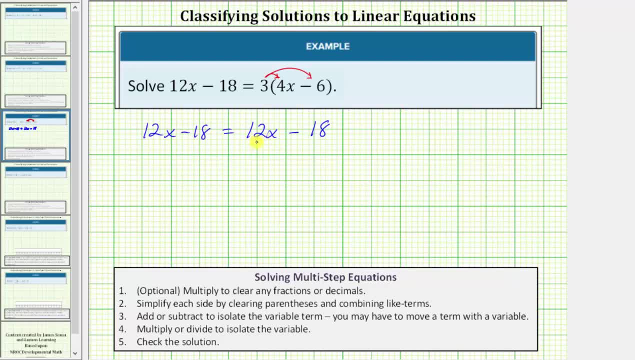 And therefore there's an infinite number of solutions to this equation. But if we didn't notice this, the next step would be to add or subtract, to isolate the variable term. Remember, our goal here is to isolate the variable and right now we have variable terms on both sides of the equation. 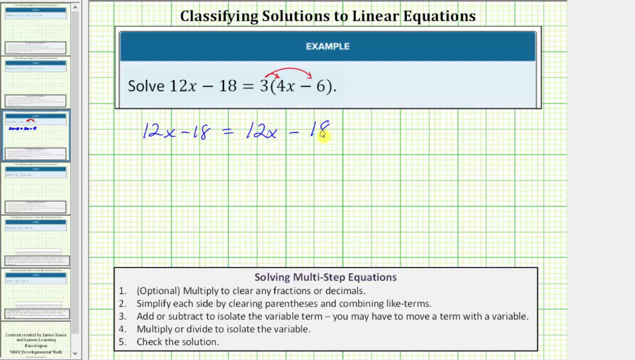 So if we wanted to undo the positive 12x on the right side of the equation, we would subtract 12x on both sides. So let's go ahead and do that. And now we simplify. On the left side, 12x minus 12x is 0.. The left side simplifies to negative 18.. 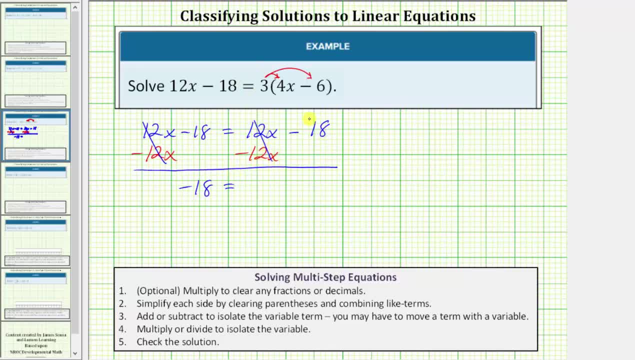 On the right side we have 12x minus 12x, which is 0. The right side also simplifies to negative 18.. So notice, in the process of isolating the variable, the variable terms simplify out and we're left with the equation: negative 18 equals negative 18.. 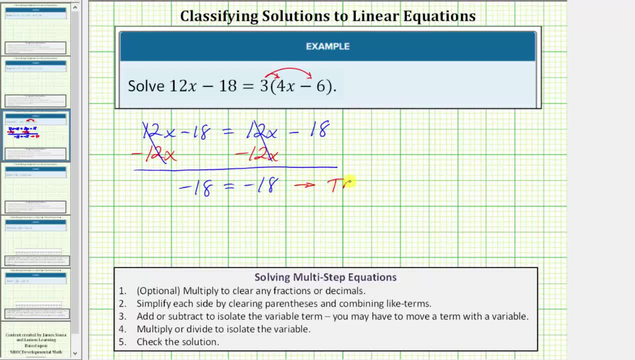 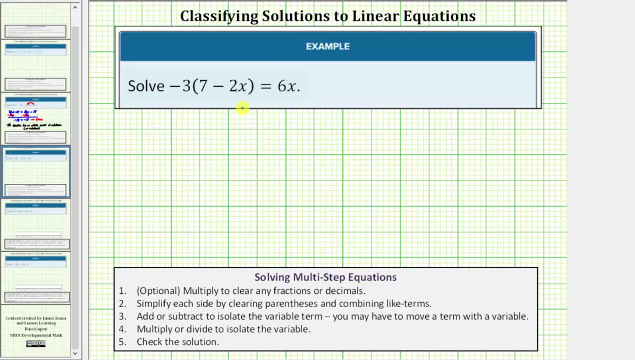 Because this equation is true. this indicates the original equation has an infinite number of solutions And, for short, sometimes you'll just see infinite solutions. Let's look at a second example. Here we have the same type of equation. So for the first step we clear the parentheses by distributing negative 3 on the left side.